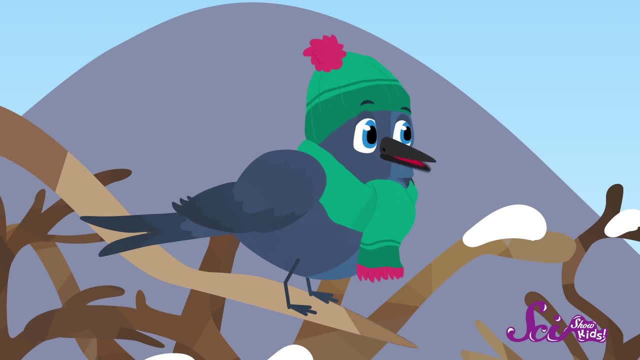 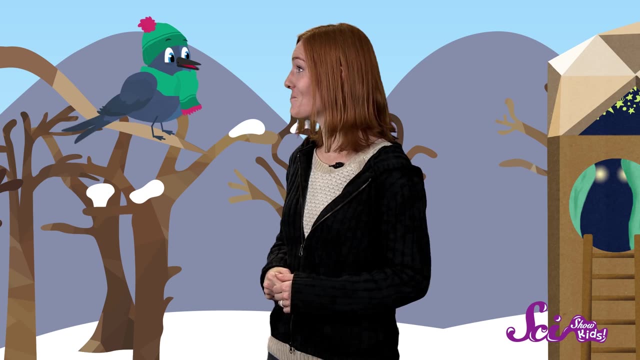 water in bird baths so they have something to drink. That would be great. I love it when people leave me snacks, And there's something else you can do too. Do you know what season comes after winter? Dino Spring, That's right. And do you know what spring brings? 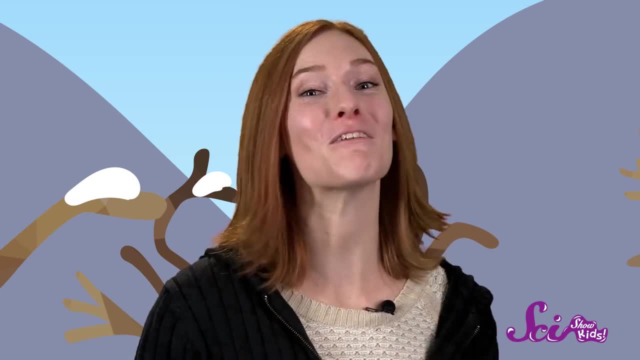 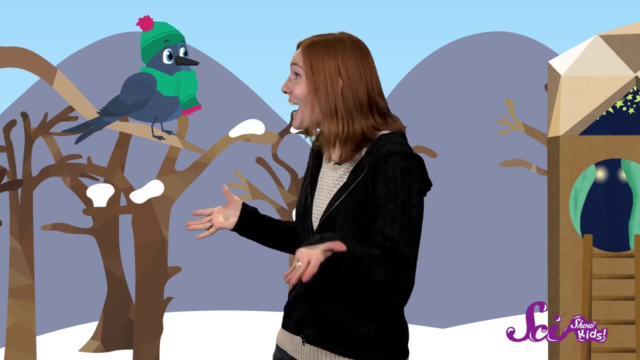 I do. Baby birds, Chicks- Yes, In the winter, birds have to get ready for their chicks to hatch And the first order of business is to make a place to lay their eggs- A nest. Yeah, Some birds start building their nests in the winter, so they're ready to lay their 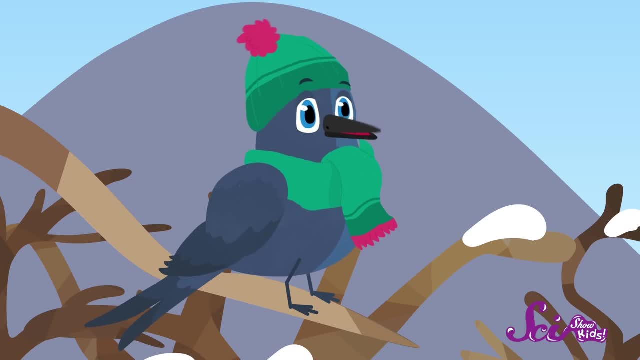 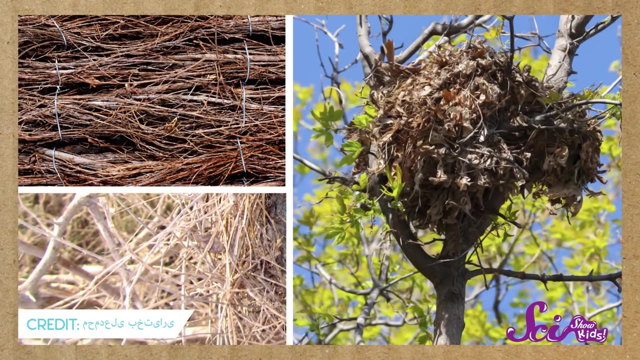 eggs in the spring, Dino. how do birds build their nests? Well, different birds can build their nests using different kinds of things that they find around them. Around here, many birds use things like twigs, leaves and grass, And for a lot of the year those things are pretty easy to find, But in the winter, the 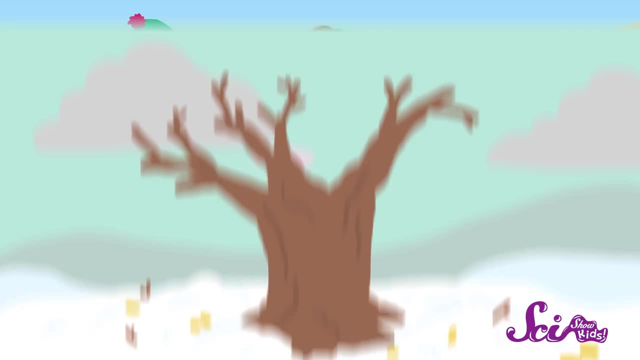 leaves have fallen and twigs and grass can be covered with snow, But that's where we can help. You can pull out leaves, sticks, pine needles and other stuff from under the snow to make a nest. Dino, how do birds build their nests? 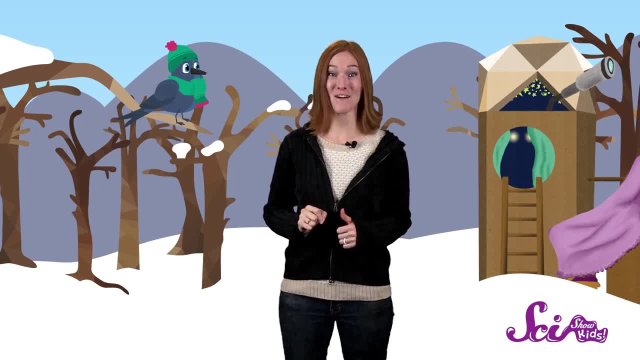 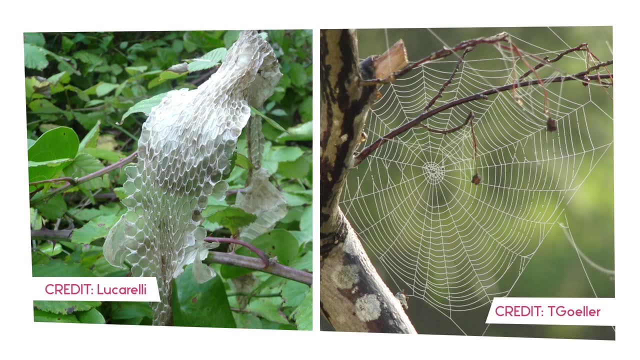 You can make them easier for birds to find and gather up, And if you happen to find something cool like a spiderweb or even a snakeskin, leave it where you found it. A nesting bird might pick these things up and weave it into their 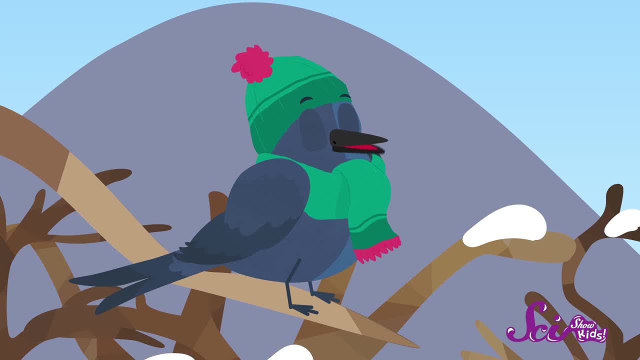 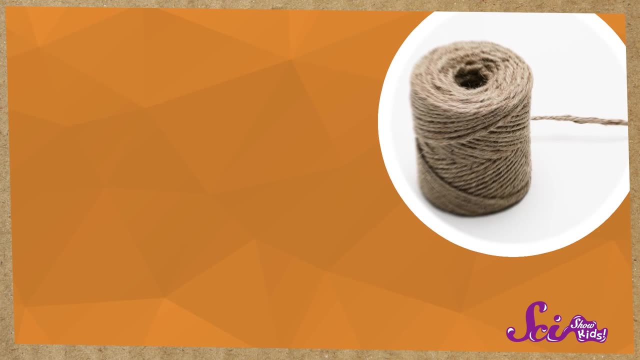 nest, Snakeskin and spiderwebs Sounds like home, sweet home, to me. Well, we can put out other stuff for the birds too. Do you have things at home that are similar to twigs and grass? What about a piece of string Or a strip of paper? 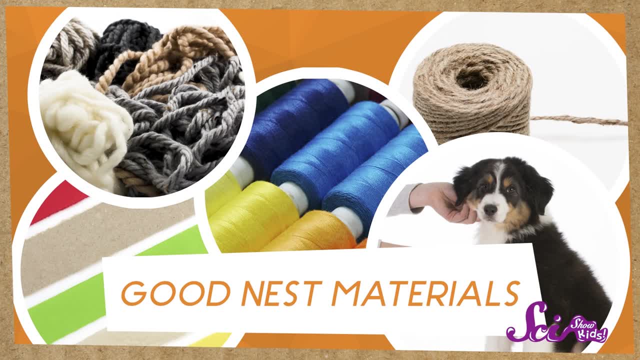 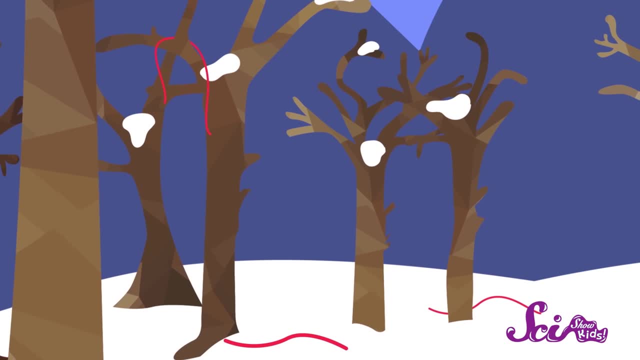 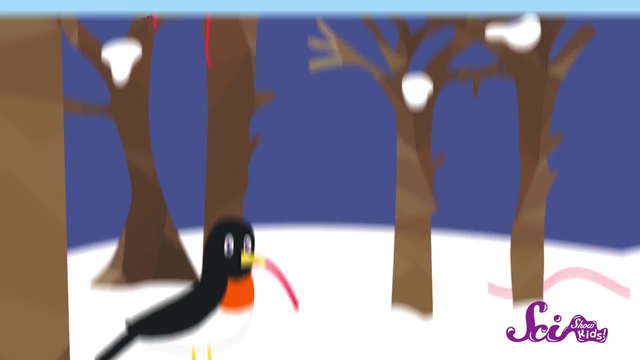 Thread yarn. even pet hair can make good nest materials. So you can put those things outside for birds. Just lay a few pieces of string on the ground or in a tree branch and then see how long before it disappears. If you're quiet and patient, you just might get to watch a bird pick it up. If you do. 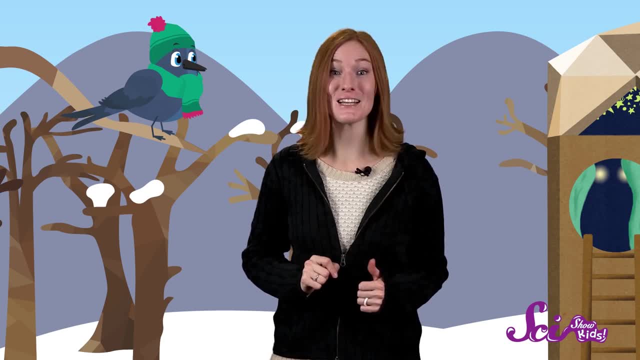 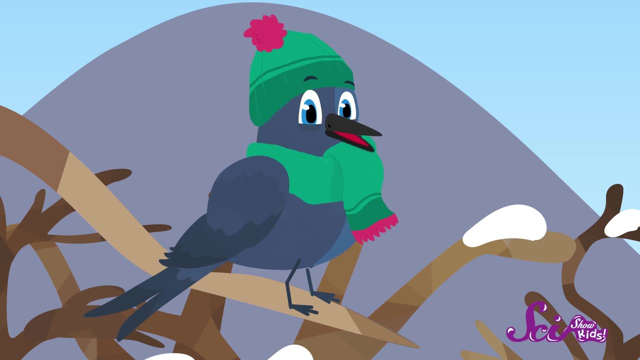 pay close attention to where the bird takes it. It may be building a nest in your neighborhood. That would be great. You'd get to do some serious bird watching and in the spring you might even get to see some baby birds- So cute. 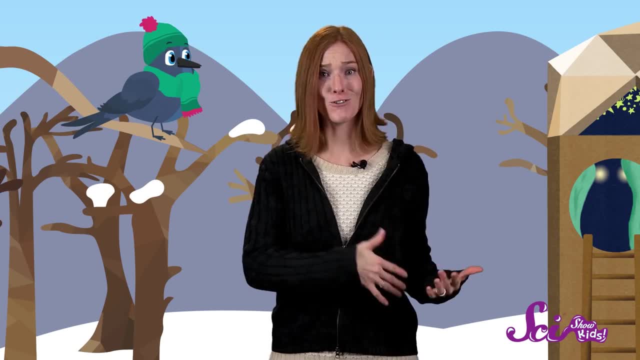 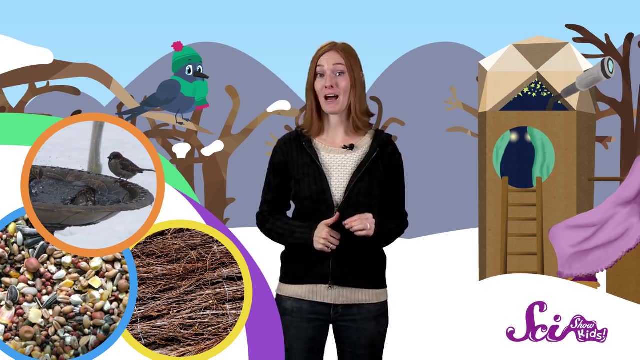 So this winter, think of the birds. They're busy, They've got to find food and water and build their nests. So if we put out a little food, water and nesting materials for them, we not only give them a helping hand or a wing, we also get the fun of watching them, And you know that.